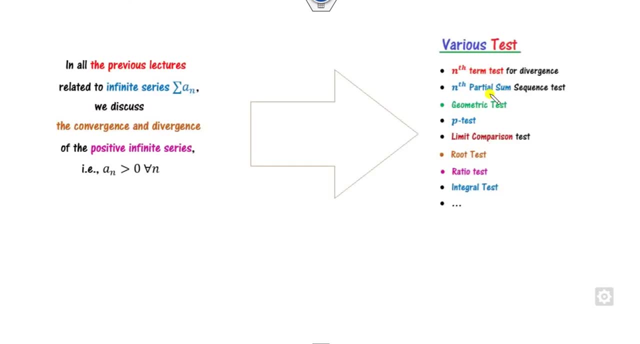 What we have discussed so far. we have discussed all those tests in our previous video which are applicable only for the positive infinite series as of here. But in this lecture we will see how you can solve the convergence nature of this alternating series. that is, minus 1 raised to power n. For this alternating series there is a test called as the Leibniz test, also called as the alternating series test, that we will discuss in this lecture. 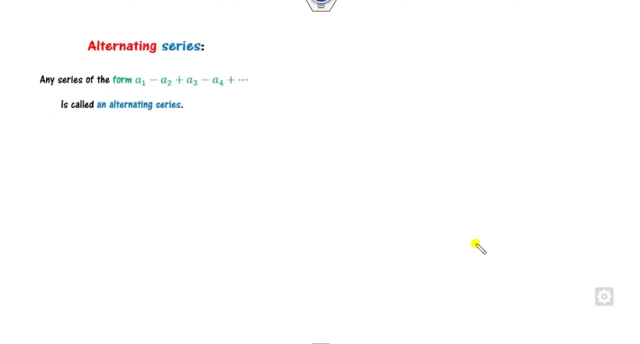 But first of all, what is the meaning of the alternating series test? Any of the series which of the form plus minus, plus minus are there, is called as the alternating series. We can express this series in terms of here: If n is equal to 1, then the first term will be my positive, positive a1, minus a2, and so on. If it is there, then again the first term is my positive, then negative, and so on, And again in this case it is a minus a1, plus a2, minus a3, and so on. So in all these case we can representing this as a alternating series test. 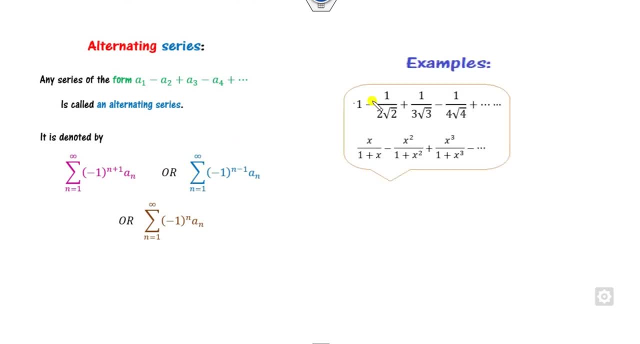 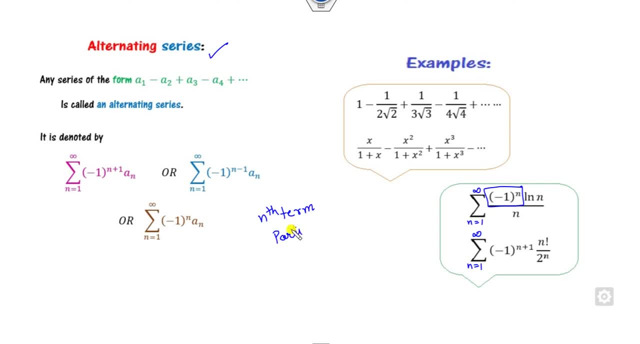 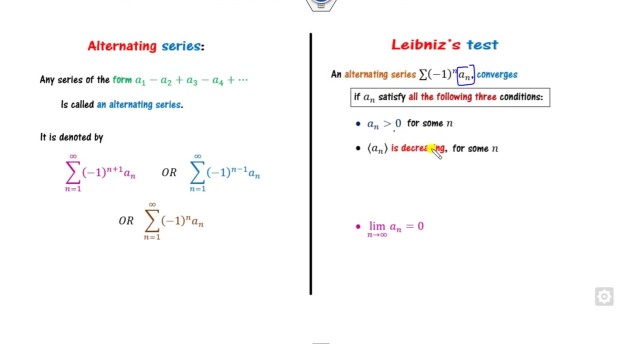 It must be the positive. It is a sequence of the a, n must be the decreasing and the limit is 0. When, any, when all these three conditions satisfied, then we can say this series is convergent. by using Leibniz test How you can prove that it's a decreasing. So we know there are the two methods. First, 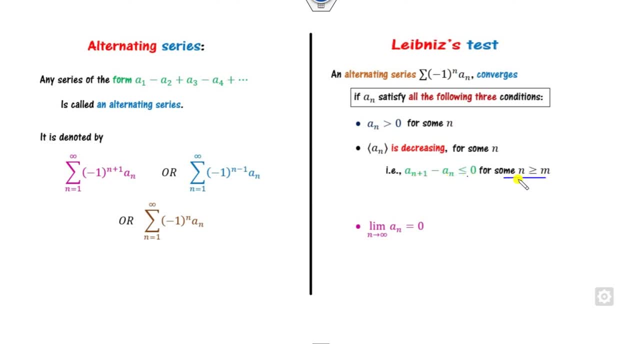 one is a n plus 1 minus of a n must be less than 0 for some n which is greater than of some numbers. Otherwise we can take that derivative and it should be less than 0. Then we can say it's a decreasing sequence If any of the series does not satisfy any at. 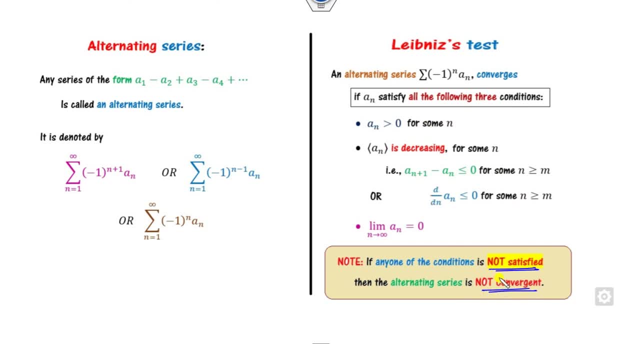 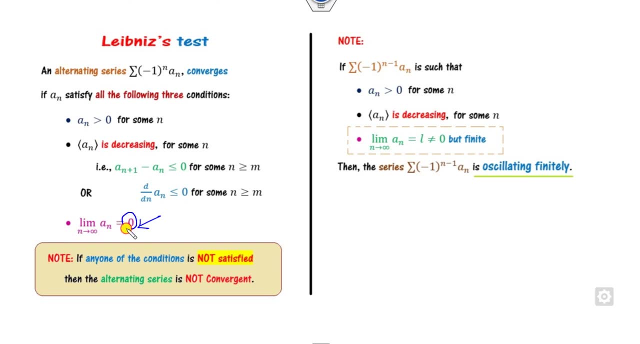 least one of these conditions, then the series is not convergent. Now, once it is here, if you look about that, if, since it must be 0, remember that it must be 0. If, instead of this 0, if it's, some say, finite number, which is non-zero, then we can say it is a oscillating. 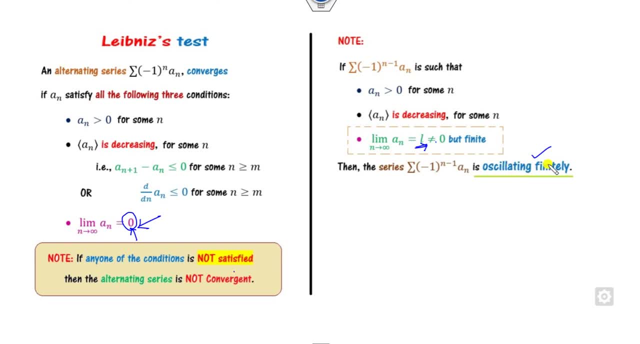 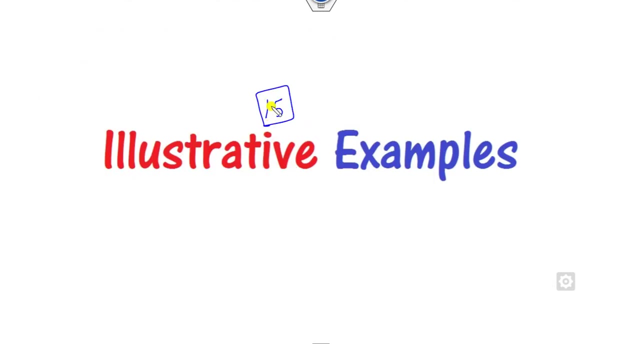 finitely series. It is not a convergent but it is oscillatory finitely series. On the other hand, if this limit is my infinite, then we can say oscillately infinitely series are. We will describe about the 15 examples in this lecture so that you can able to understand. 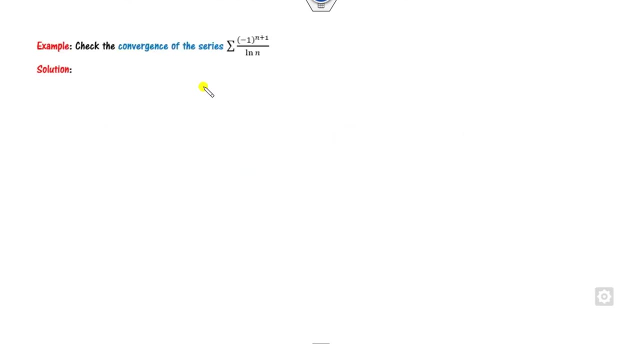 it completely this concept very easy. So look at the discuss the convergence of the series So clearly says that, because of this presence term, it is my alternating series, So we can apply this three step rule. So what is the a? n If you compare this series? 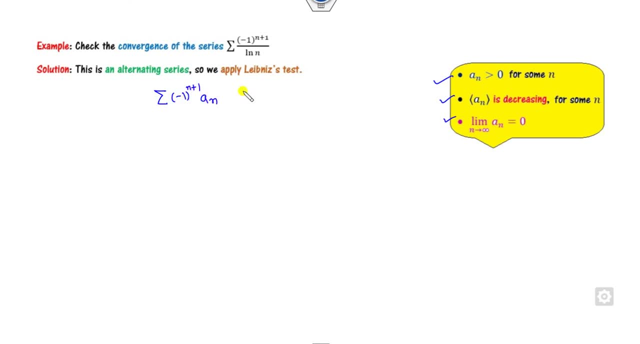 with respect to here, what is the a, n? a n is nothing but my 1 upon l n. So we can check about this nature of it. Now clearly say that what is the n is n is my natural number, So n definitely be a greater than equal to 1.. When n is greater than equal to 1, clearly. 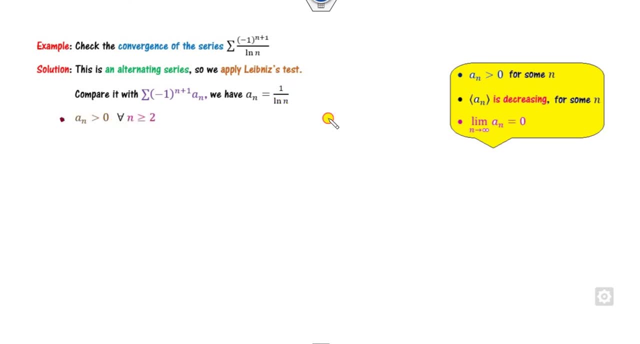 says that this number is my positive, Because when n is equal to 1, it is my 0. So 1 upon 0 is infinity, which is again a positive, But it is for some n. you can say n is greater. 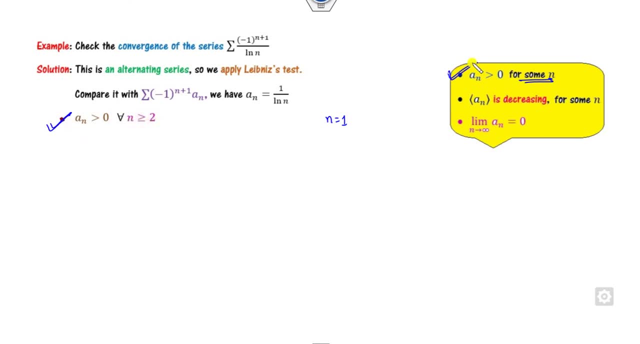 than equal to 2.. It is always positive. 1 upon 0 is infinity, which is again a positive, But it is for some n. you can say n is greater than equal to 0. This is the first condition satisfied, How you prove that it is decreasing. 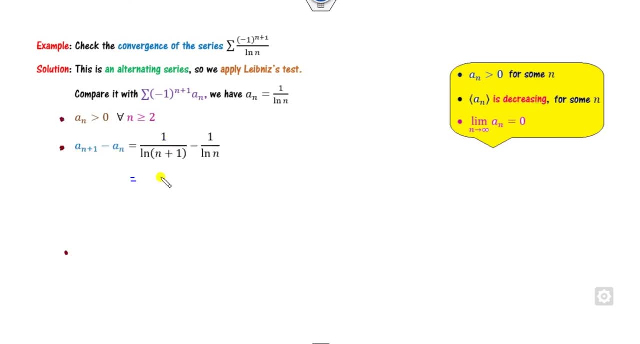 We can start with a n plus 1 minus of a n. If you solve them you can see l n minus l n of n plus 1.. So clearly says: if you look about this numerator, this part l n, because if you take n is say 1.. So this is 0.. This is my 0 minus l n 2.. So which is again a. 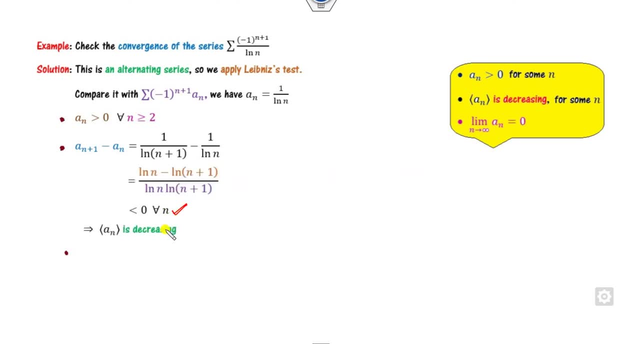 less than 0. So it is less than 0 for all the values of the n. you can also take that derivative rule. if you take that derivative of this, an, what is the derivative of this? this is a minus of this, which is again less than 0 for all, and therefore this: 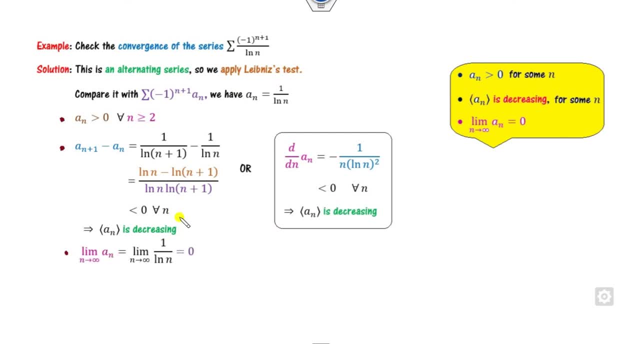 second property satisfied. third property clearly says that log of infinity is 0, so we can say it's a here. so since all these three properties are satisfied, so by using this Leibniz test, this series is my conversion. look about this next example. again, you can say it's a minus plus and 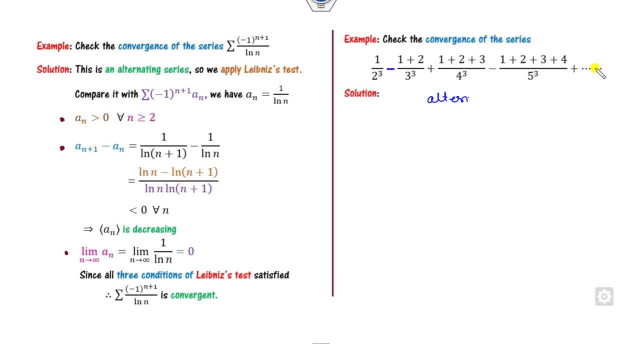 then so on. so which is an alternating series. what is the nth term of this? you can say: what is the how you can write this? this is the minus of this. so the first term is 1, 2 and so on. so I can say: a n is nothing but 1 plus 2, up to n, and here is n cube. so 1 n is 1, it is a 2, so it is n plus 1. 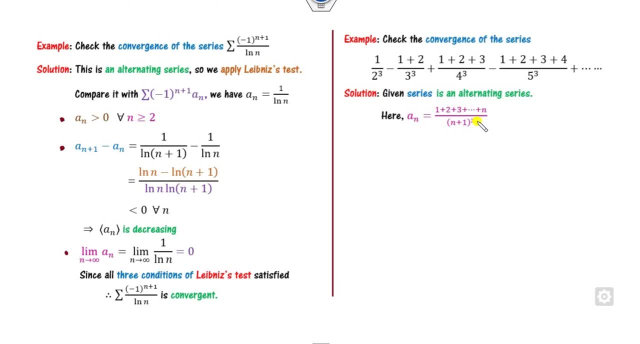 whole cube. this is my nth term, so what is the numerator is? you can say this is a, g, ap series, so the sum of the ap series, so the sum of the ap series. so the sum of the ap series I can return like of this, now it will be 1 is cancelled out, so the series becomes my here now. 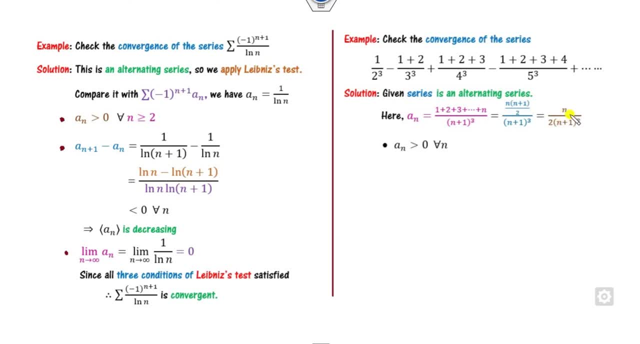 we can check about these three properties. for this clearly say that for all the natural number, this number must be greater than 0. how you can prove the decreasing? you can start with here, or you can take the derivative as per your convenient. you can take the LCM, you can see, it's a minus n square. 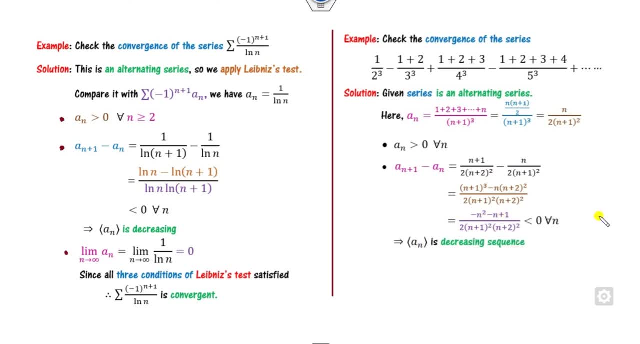 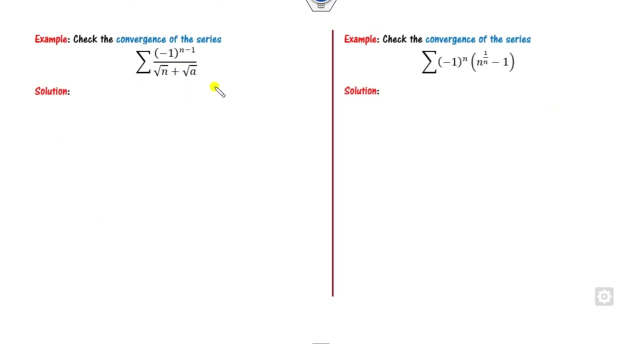 which is always less than 0 for all the values of n. what is the limit? you can clearly say that this is the number which is less than 0, because if you multiply this by infinity- by infinity we can apply the allopator rule- we will get as a 0. so therefore, series is by convergent. by using Leibniz, test you. 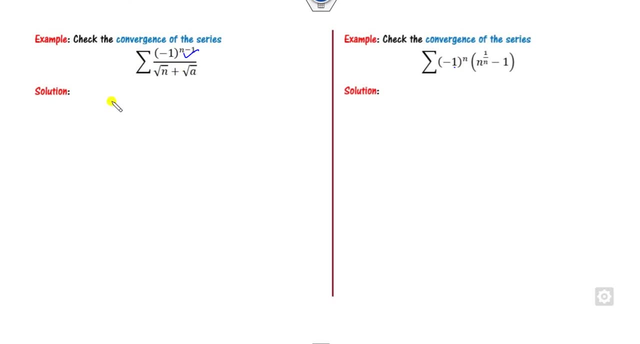 can see. both the series are my alternating series, so there is only one test, called as the Leibniz test, applicable in this case. what is the a? n is 1 upon this, so, which is clearly a positive number, because in this case a must be the positive, because otherwise root of a is complex number. how you can? 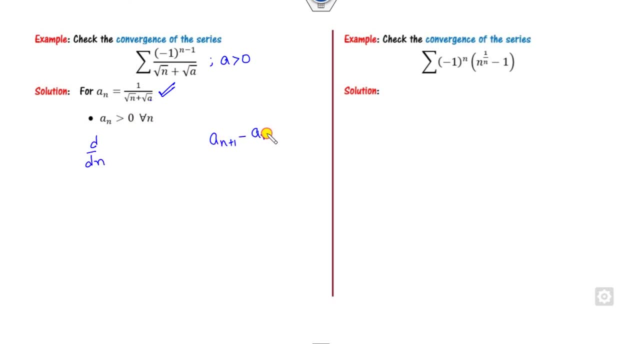 calculate of which is effective. so, abnd, we can take the derivative and we will get this confluent and in this case, thenik of the derivative, or you can take the an plus minus an, so you can take like here. so clearly says that this number is a less than 0 for all n, hence it's a decreasing, if you. 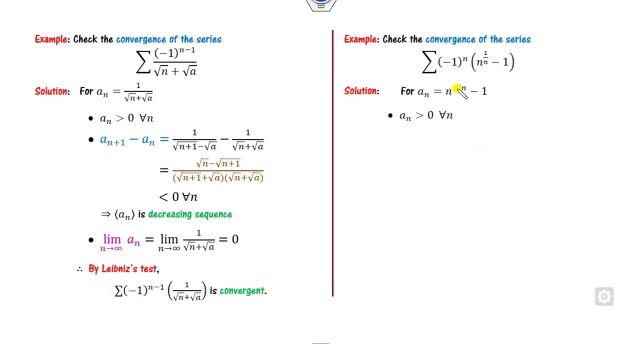 take this third property that is a limit and approaches infinity, which is 0, so clearly say that by Leibniz test is a convergent. in this case, what is my an, an is nothing but my n raise power half, which is clearly a positive number. 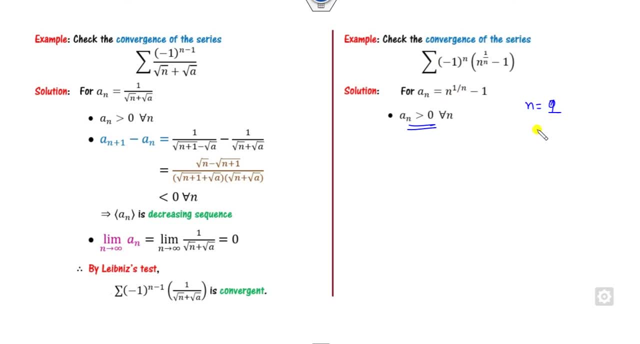 number, because when you take n is 1, it's a 0. when you take n is 1, then it's a 0. when you take n is 2, then it's, which is again a positive number, and so on. you can take the derivative because it's. 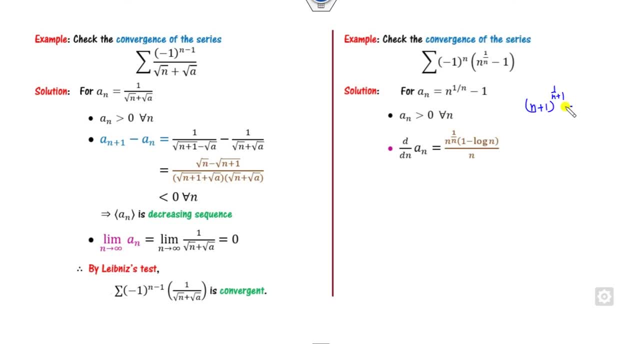 it's- sometimes it's not possible to find this as of here- which is a n plus 1 minus of a n, so either you can solve like this way or you can take the derivative which is here. clearly says that this number is my less than 0, for n is greater than equal to 2, so because what? 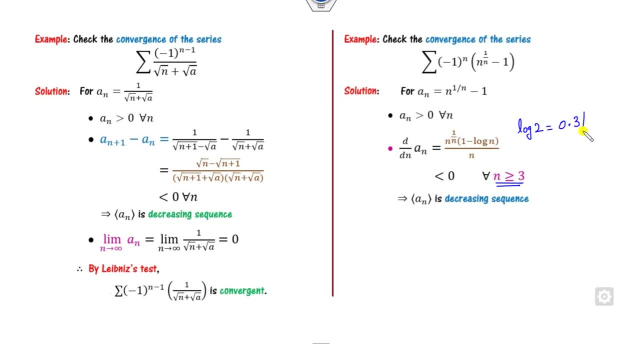 is the log of 2, that is nothing but 0.3 or 0.6 are there, which is a positive number, so which is whenever n is greater than 3, it is a positive, it's a less than 0. also, you can say: limit what. 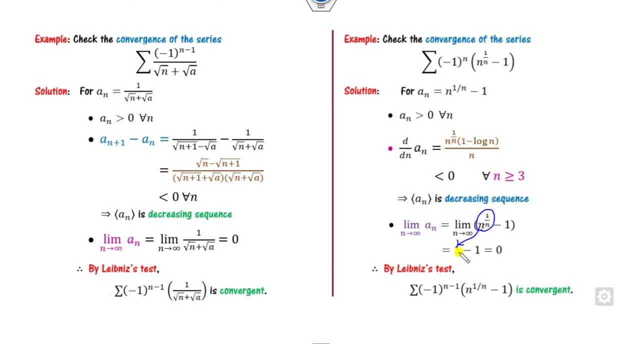 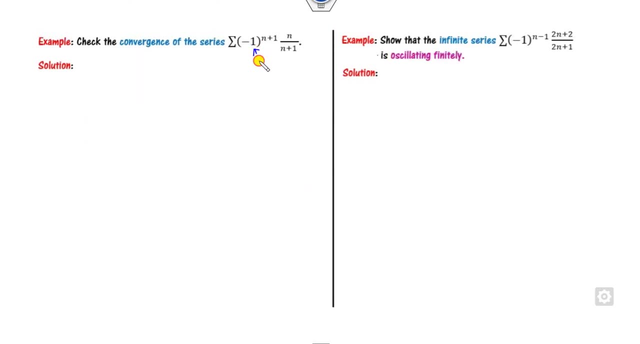 is the limit of the n raised to power. 1 by n is always be the 1, so 1 minus 1 is 0. so therefore limit test is a converging series. again, this is a alternating series, so we can apply this one- a n is my here- which is clearly say: 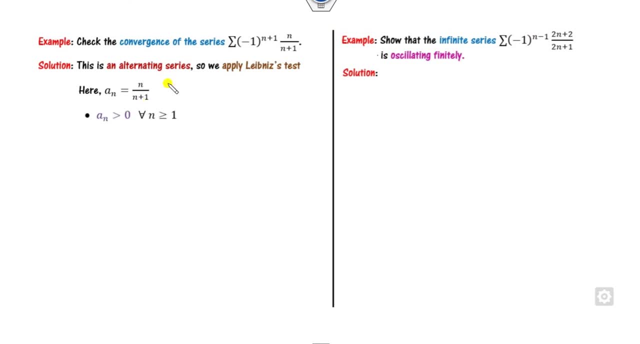 that it is a greater than 0, the first property satisfied. we can take the second property either. you can take the derivative. derivative is my minus, because this number is always positive. so due to minus, it's a less than 0. what is the limit? limit is my 1, which is a non-zero. what is the 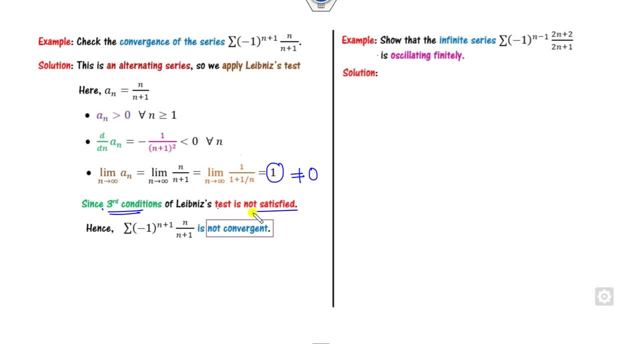 meaning of that. it means the third condition of the Leibniz test is not satisfied. therefore series is not convergent. remember at least one of the condition violated, then it's not a convergent. but we already discussed that. if this limit is a non-zero but a finite, then we: 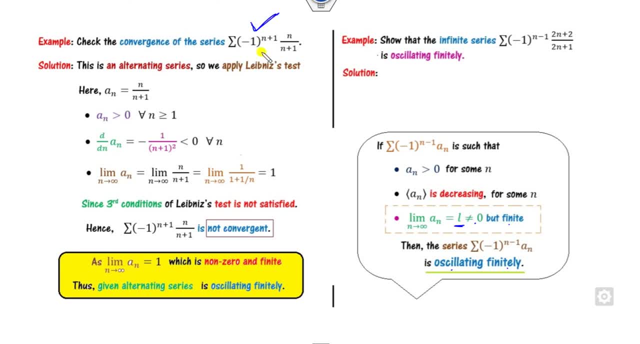 call as the oscillatory finite series. it means this series is my oscillatory finite series because they are check about the convergence of the nature. similarly, for the second part, again, this is my a? n. you can write this number as here, which is clearly greater than 0. 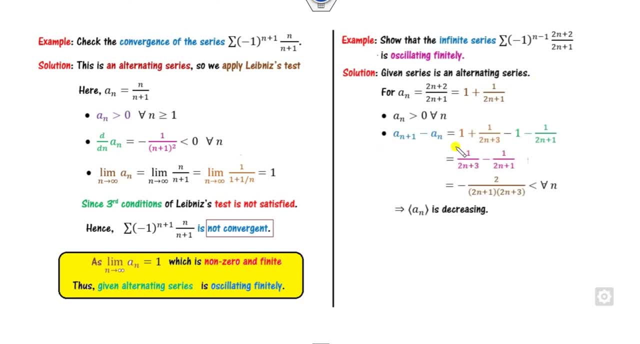 because property satisfied, you can take the a n plus 1 minus a n, so this will be canceled. you can see that if you take the lsf because of this minus, it will be my less than 0 for all n. if you look about the third property, what is the limit of this? it's a one which is a non-zero. it means it is not. 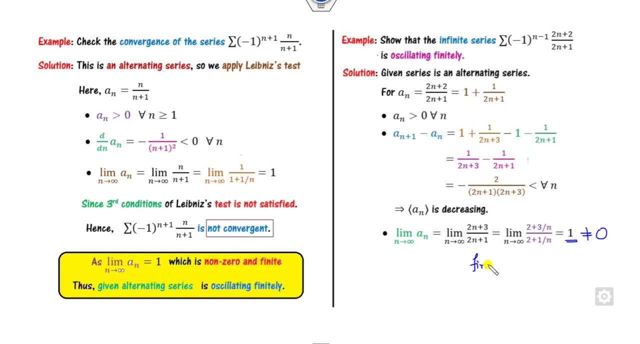 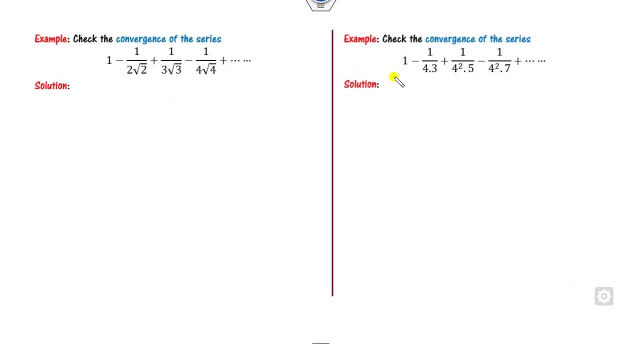 convergent, but you can see which is a finite. so therefore, by using the property, we can say it's a finitely oscillate, goes to the infinity. then we can say it's a infinitely oscillate. again. you can see, these are my alternating series. how you can say, how you can write that I can write this number as first number. 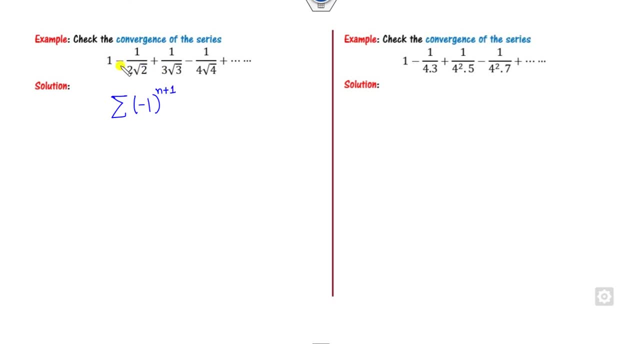 is my positive, so I can write as n plus 1. so what is the nth term is the numerator is my 1, 1, 1. I can write this number as also. so what is that? this is here? this is number and start from the 1 to infinity. 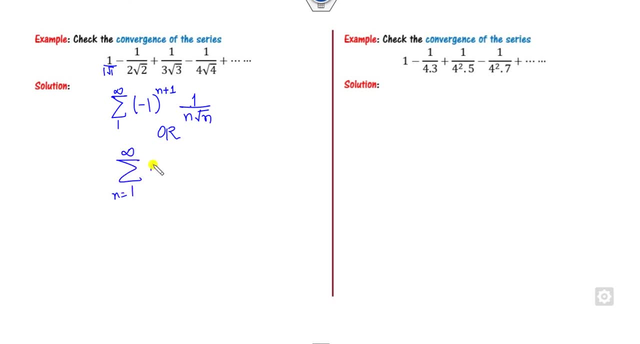 also write this number as 1 to infinity and is minus 1 raised to power: n minus 1. that is the same thing for here. again, this will give the first number as a positive. so the a, n is my here. clearly say that this number is my positive for all: n. this is the decreasing sequence because this number is 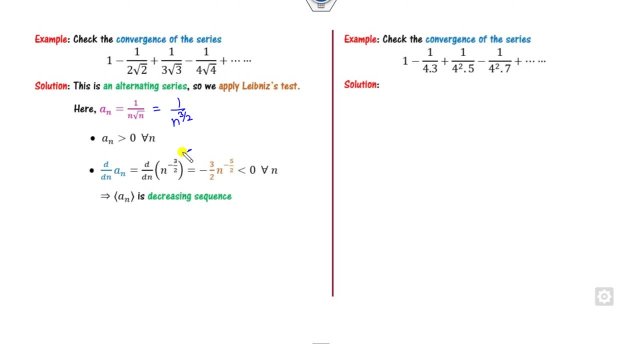 my 1 upon n, raised to power 3 by 2, which is a decreasing sequence. also, the limit is my 0, so therefore it is my convergent how you write this one, so I can write this number in terms of 4 raised to power 0, 3. there is a odd series 1 earlier, so 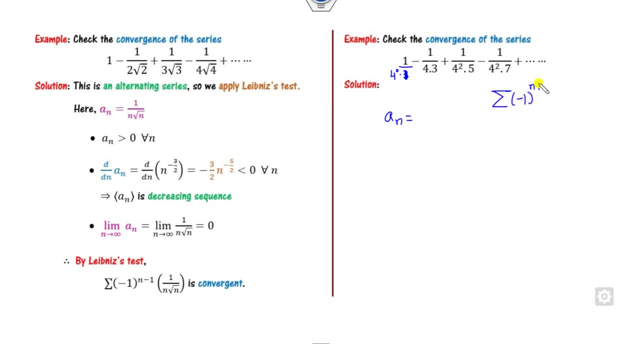 what is the nth term? I can write this number again: n plus 1 of a? n and start from the. so what is the a? n? the numerator is: my 1 denominator is 4 raised to power 0, 4 raised to power 1, and so on. so it is: 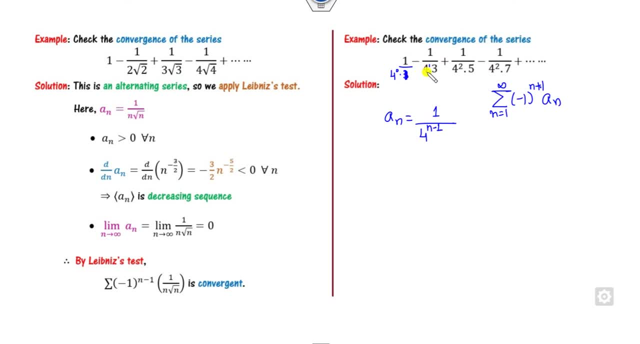 n minus 1, because the first term is 0. then here is 1, 3, 5. this is my odd series. okay, so this is again AP. you can write that AP a plus n minus 1 into D. that is the first term. common difference is my 2, so 2 n minus 1. this is my a? n of this series. now clearly say that this is number. 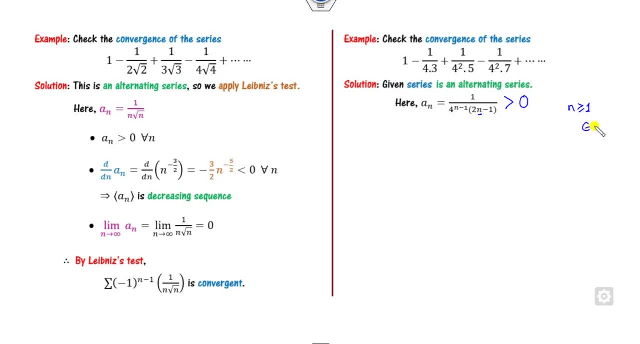 of my positive. given this n is my greater than or equal to 1, belongs to natural number. this number is my positive. this number is my positive. you can. Can you take the derivative of this? yes, It is not. you can take as a u upon v, but it will take some lengthy procedure. 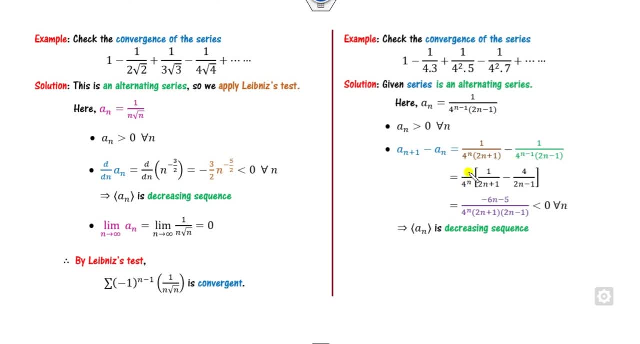 Best way that you can take as a a n plus 1 minus a n. I can take this comma. Now you can see this number is always less than 0. It is decreasing. What is the limit? You can say it is a 1 upon infinity. 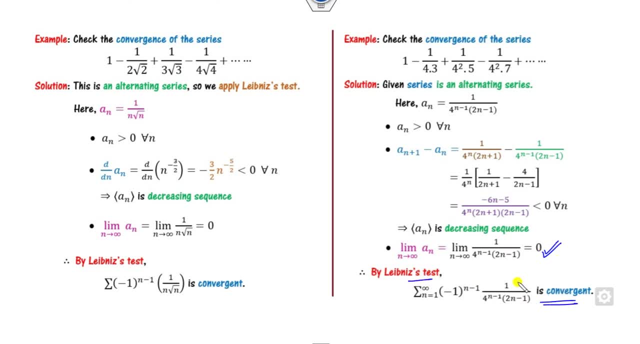 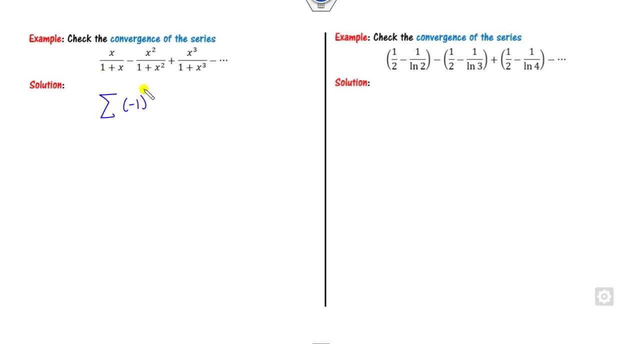 That is a 0. So by limit test it is a convergent series. Look about the another Again. this is an infinite series which is alternating, So we can write this as n plus 1.. What is that? 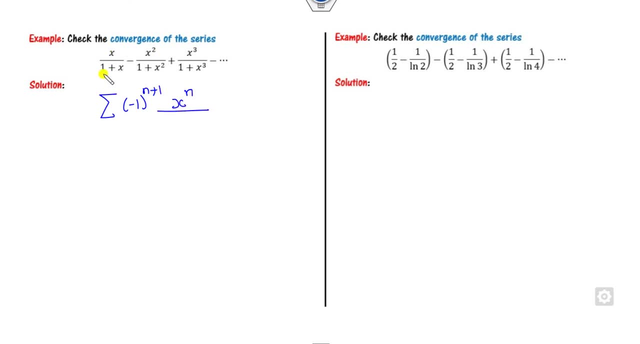 This is x, x square x cube. This is x raised to power n: 1, 1, 1.. This is x plus x square plus x cube, So I can return as x raised to power n. This is 1 to infinity. 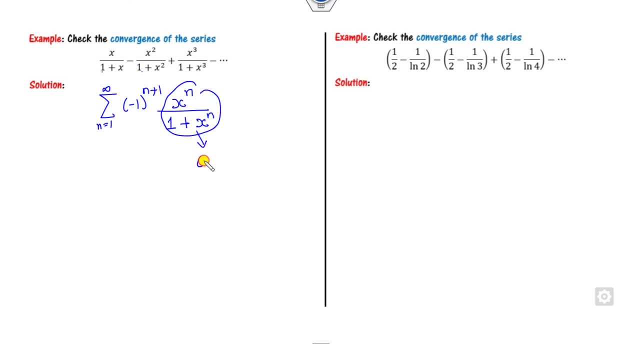 So this is there, So we can say this number is my a- n and we can check for the alternating series test. This is positive. You can take as a ratio. Now you can say this number is less than 0 only when x lies. 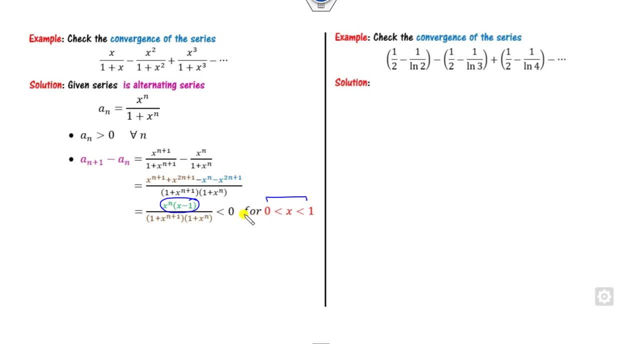 Between 0 and 1.. So therefore, this series is decreasing only for the x less than lies between 0, 1.. Clearly say that why it is a 0? because whenever x lies between 0, 1. Whenever x lies between 0, 1.. 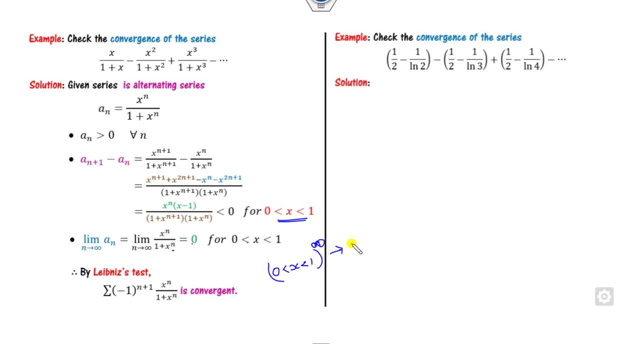 So anything power of n as n approaches infinity goes to the 0. So this is a 0.. How you write this series? I can write this number as first number is positive, So n plus 1.. So 1 by 2,, 1 by 2, everything is common. 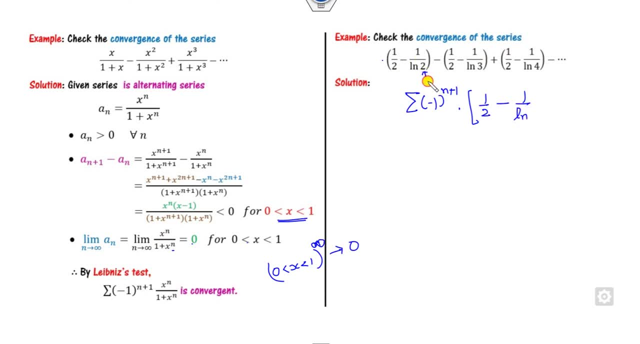 So it is 1 over ln. The first term is my 2.. So it means I can return as n plus 1 and start from the 1 to infinity. Or you can write this number also as n. 1 by 2 minus 1 over ln of n. 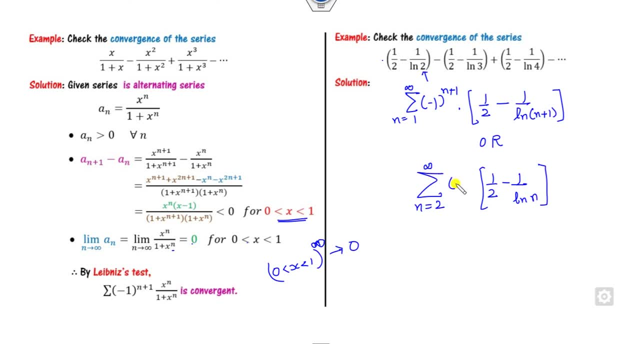 But then you can start from the here as a 2. Then in that case your first term is a positive. Then instead of this n plus 1, you have to write this as a n, So both have the same. That is on your choice. 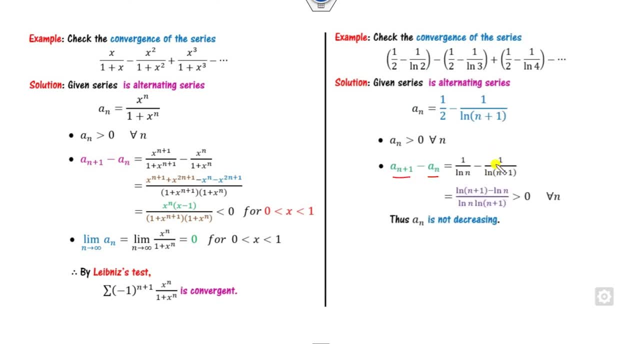 Clearly say that it is a positive number You can take as in difference. Clearly say that this is always be greater than 0. So it means it is not decreasing So once. what is the meaning of that? The second property is not satisfied. 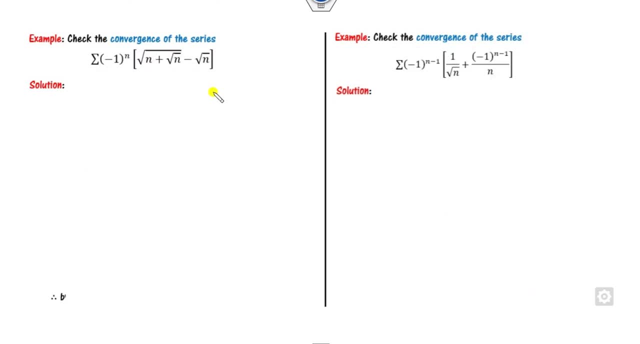 Therefore, series is not convergent. Again, this is alternating series. We can check for the an, We can check for the derivative or for the decreasing. Clearly says that it is a decreasing or increasing. Look at What will happen if n is 1?. 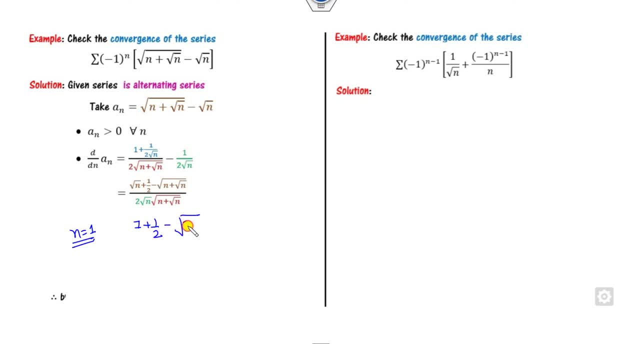 So it is 1 plus 1 by 2. It is 1 plus 1: 2.. So that is a 3 by 2, minus of root 2, which is less than 0. If you take n is equal to 2.. 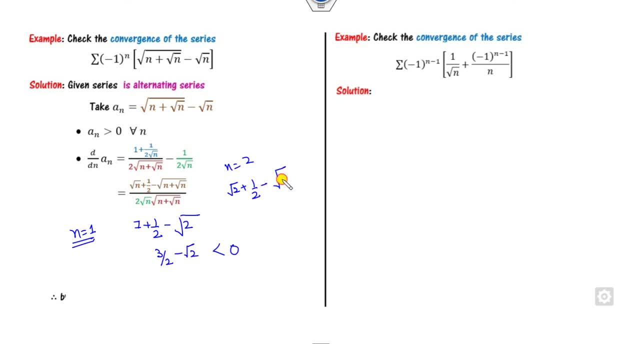 So it is my root 2 plus half minus 2 plus root 2.. So clearly say that it is a root 2 plus half. This number is always be less than 0.. Look for the third condition. If you take as a limit as n approaches infinity, you can summarize, you can rationalize them. 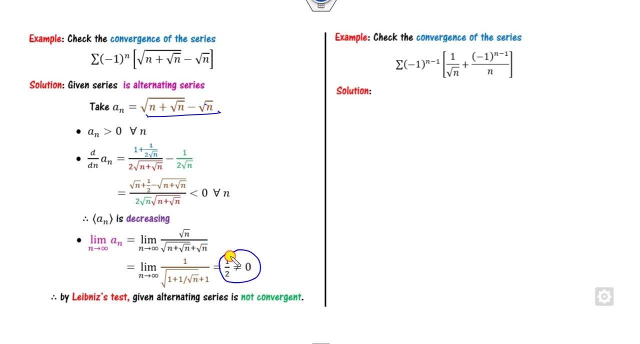 You will get as here, which is a non-zero. So third property is not satisfied, So it is not convergent. Look at that Now. there are the 2 of minus 1 are there? So firstly, we can open this summation. 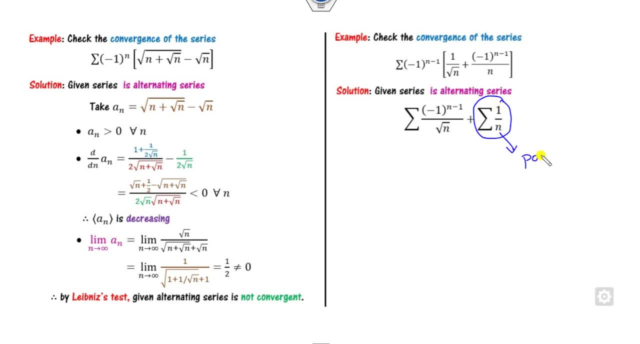 Now, in this case this is a positive series. So clearly say that this is a positive series. It means you cannot apply this Leibniz test for here Because it is not an alternating. So once it is not an alternating series, you can't apply the Leibniz test. 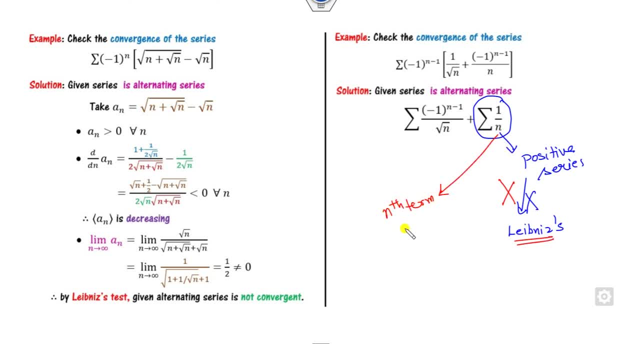 So which test will be applicable here? You can apply the nth term test, You can apply the p test, You can apply the ratio test, You may apply for the root test, and so on. So clearly say that this series is my divergent because of the p test. 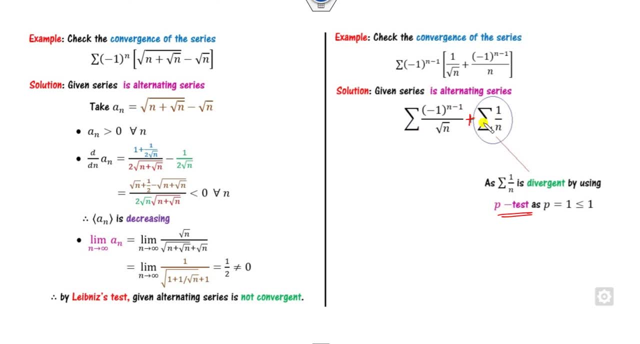 So it's a plus sign or minus sign whenever at least one of the series is divergent. The complete series is my divergent. However, if you look at this, If you look about this series, it's a negative series, it's an alternating series. 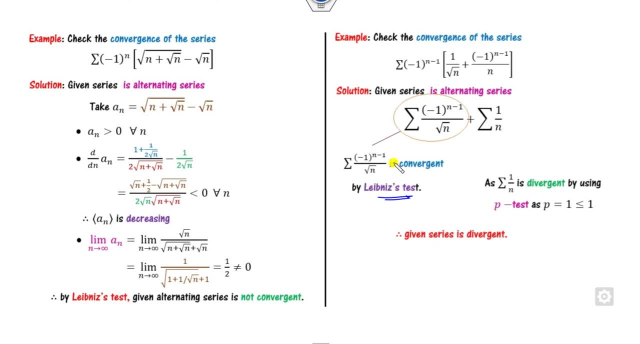 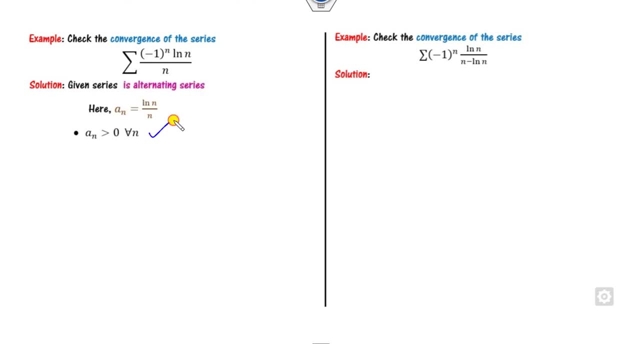 So you can apply as a Leibniz test which you can see, that it is my convergent. Look at the second, last examples are there, which is again given to you here. You can start with the derivative. You can see which is a less than 0 for all n which is greater than of e. 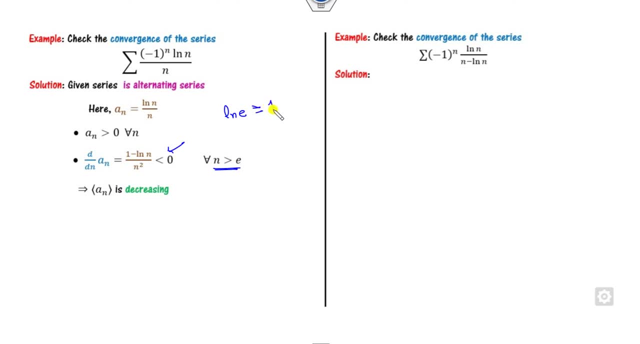 Why? Because ln of e is my 1.. Again, you can see the limit is my 0, which is convergent by Leibniz test. So if you look about this example again, this is a positive. you can take the derivative, which is again the less than 0 decreasing, and you can take the limit, which is a Lopeter rule. you can apply that and you can say it's a 0, it's a convergent series. 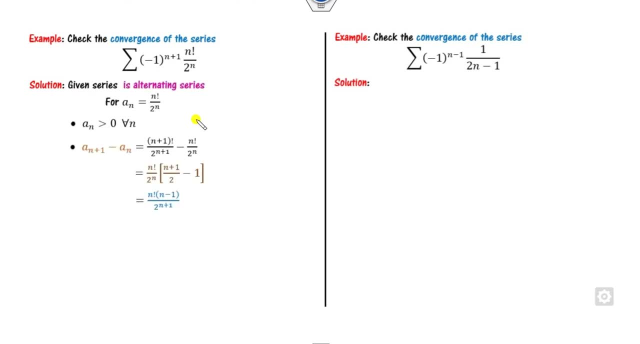 Again, this is a very simple example. you can see whenever an is here, which is always positive, you can see an plus 1 minus an. you can take as a common. you can see This number is always be positive whenever n is greater than or equal to 1, because it's n minus 1.. 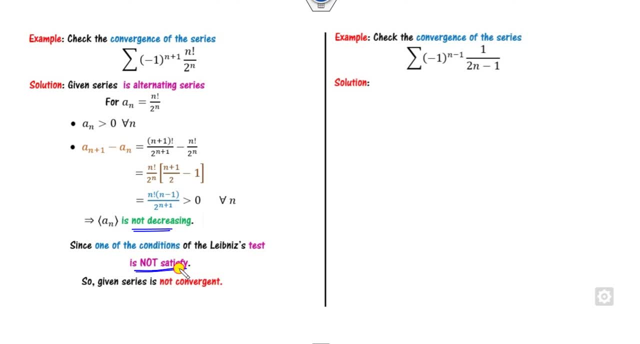 So it means it is a non-decreasing, So condition is not satisfied, the series is not convergent. Look about this one which is positive series. Clearly say that it's also the decreasing. Also you may take as a derivative. 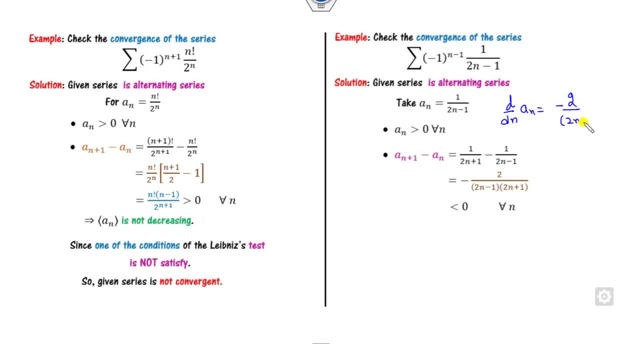 What is that derivative is my here? This is minus of 2, 2n minus 1 whole square, which is my less than 0.. And the limit itself is 0.. So it is a convergent series. Some questions are excised for you. 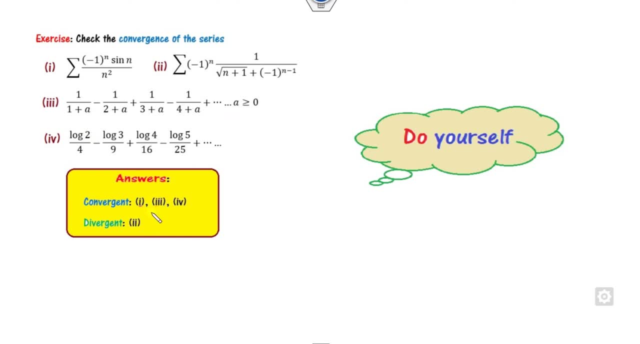 You can do it yourself. These four questions are there and these are the answers. Some more questions are given to you. You can try to solve it with the help of this Leibniz test, so that you can able to understand this concept more clearly.